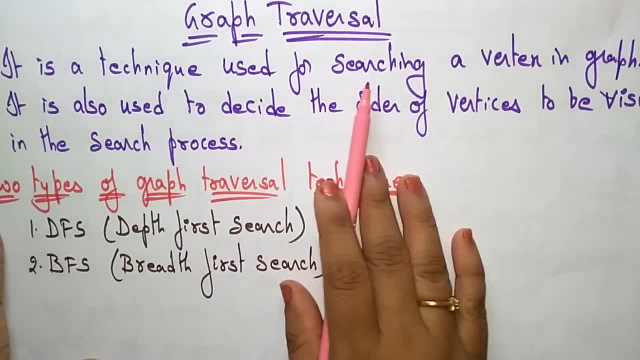 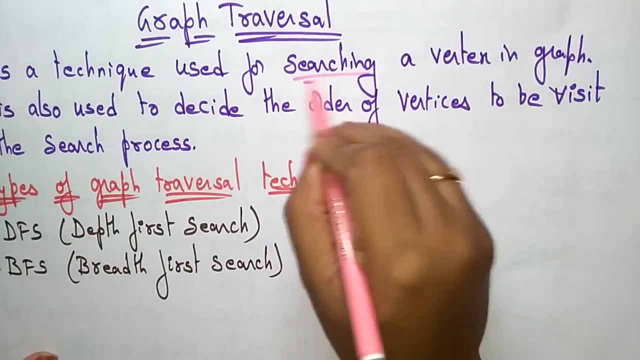 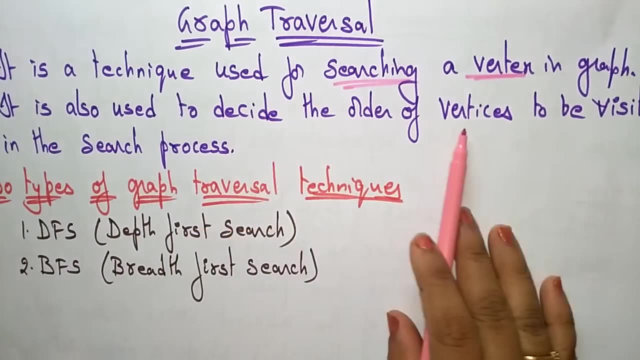 explain a graph. traversal is a technique used for searching a vertex in a graph. so we have, this is one of the method for searching a vertex. the main thing is we are going to search for a, a particular vertex in the graph. it is also used to decide the order of vertices to be visited. 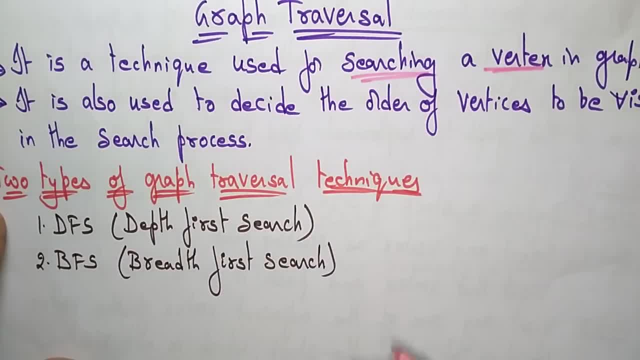 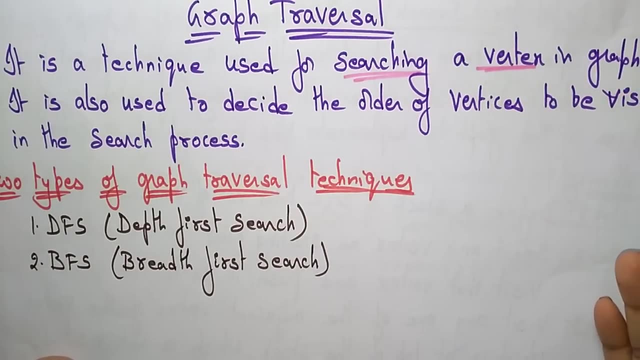 in the search process, the graph traversal. traversal means we are going, uh, visiting the nodes, visiting the vertices. so this graph travels is also going to decide the order of vertices means first which vertex we are visiting and next which vertex we are visiting, so it decides the order of the vertices to be visit in the search process. 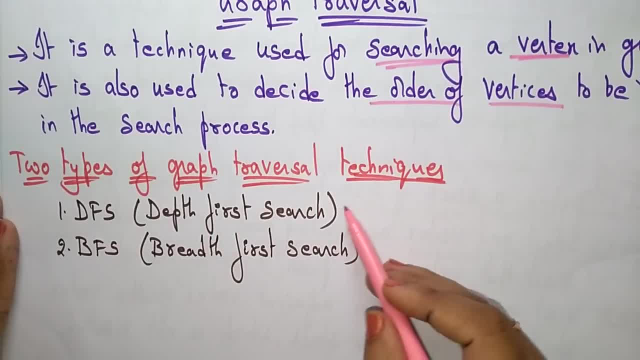 there are two types of graph traversal techniques were there. one is the breath depth first search and the breadth first search. so actually we had already seen what is the dfs and bfs and different topics when we are discussing about the trees and when we are discussing about the stacks and the use. okay, uh, now let us see how the graph. whatever the graph, 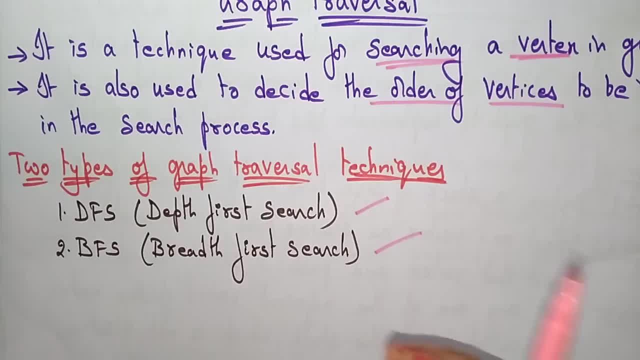 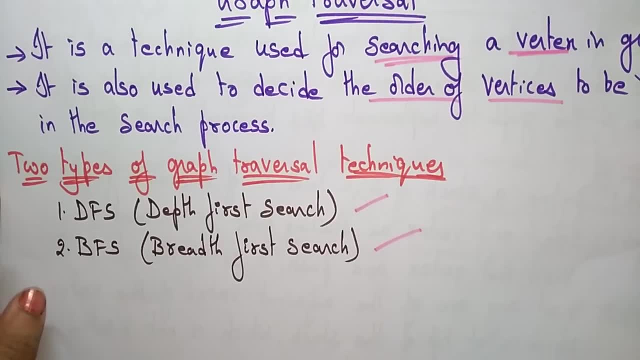 that is there. so the graph in the graph we are. we want to visit the nodes. if you want to visit the vertex, you, you can follow two techniques. the visiting of the vertex can be done in means. searching of the vertex in the graph can be done in by using two techniques of graph travel cell. 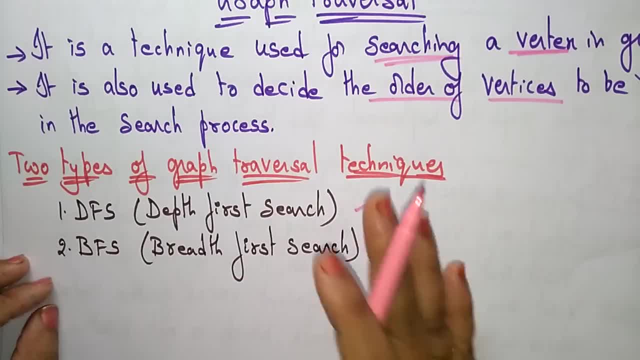 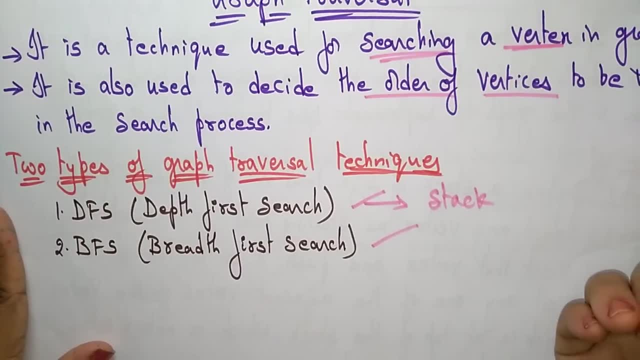 either you can follow depth first search or breadth first search. the main difference here is: dfs uses a data structure of stack for storing the values in the form of stack, and here bfs uses the data structure as a cube. so this is the data structure of the stack, and here bfs uses the data structure as a cube. 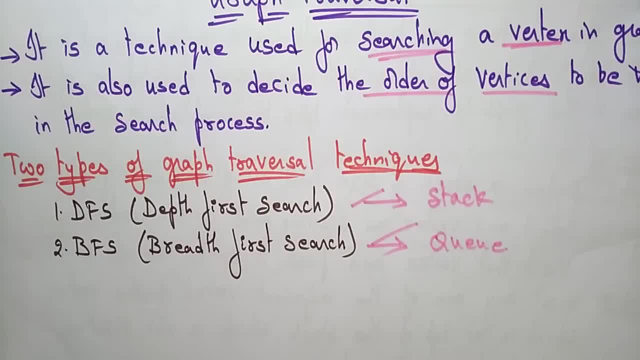 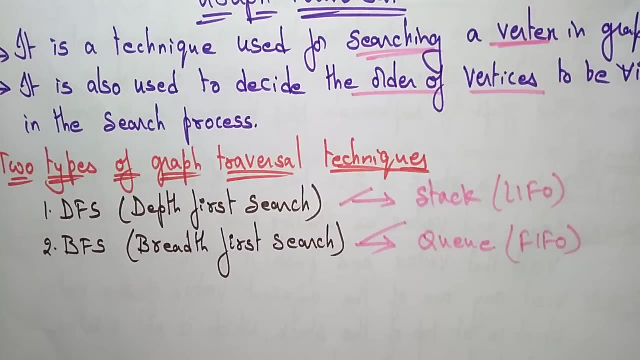 there is a only difference: the way you are visiting and deleting the nodes from that memory. it's in the form of stack and the queue. stack is last in, first out and whereas queue is first in, first out. by using these techniques, we will implement the dfs and bfs. now let me 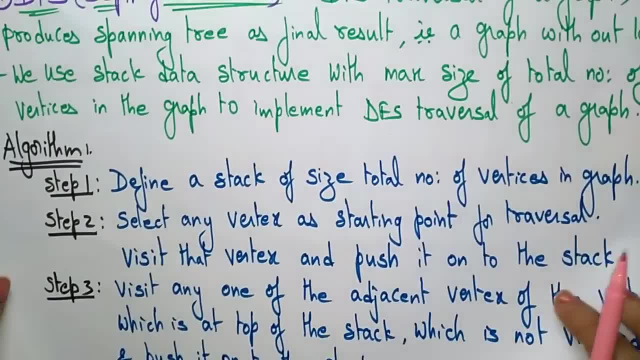 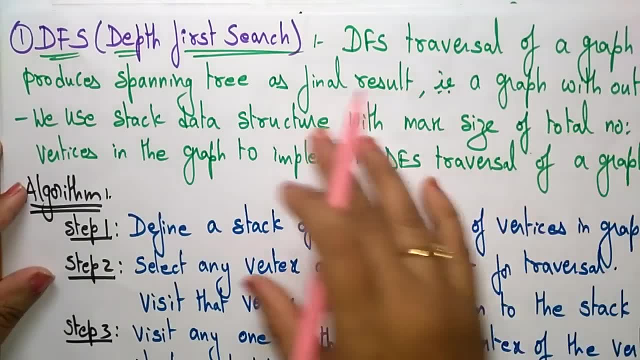 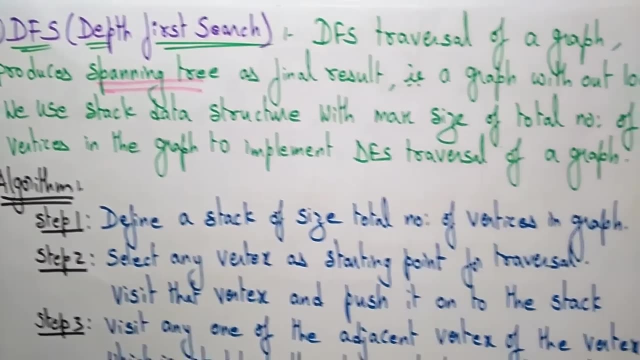 explain about dfs. dfs is the depth first search, the depth first search. traversal of a graph produces a spanning tree. so spanning tree means which is not completely connected, means it's open, whereas the graph is a complete connected graph. you it is. all the vertices will be connected. 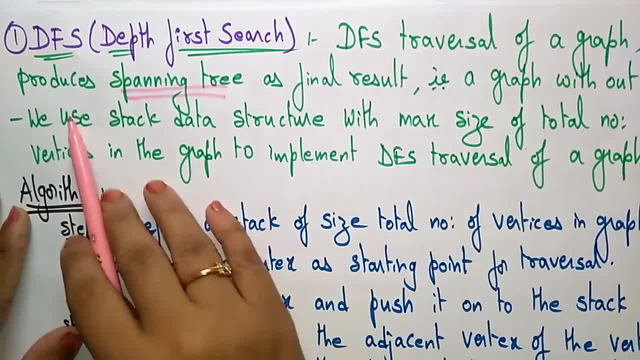 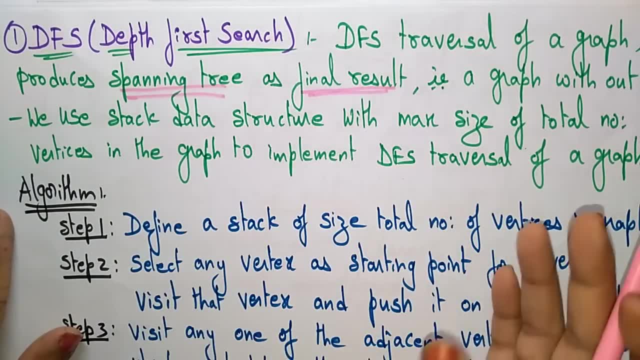 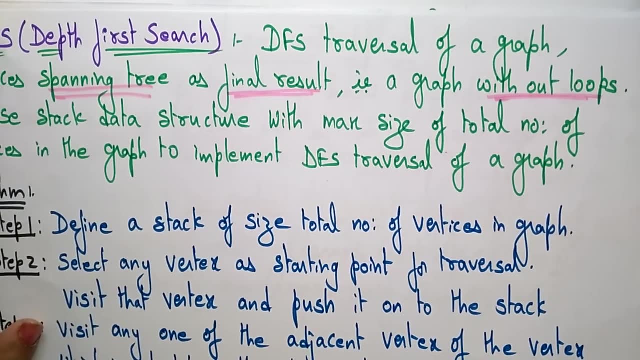 the depth. first search traversal of a graph produces a spanning tree. as a final result, whenever you are visiting all the nodes, it produces the output as a spanning tree. that is a graph without loops. spanning tree is nothing but a graph without loops. you call it as a spanning. 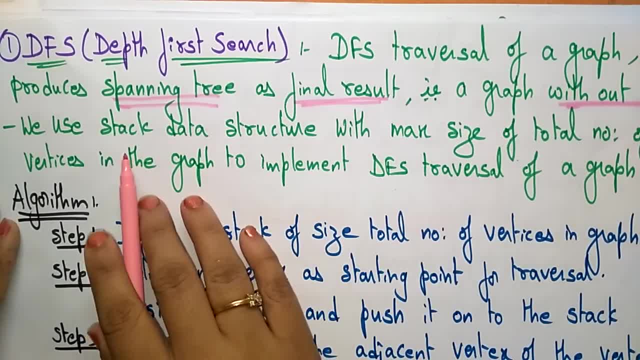 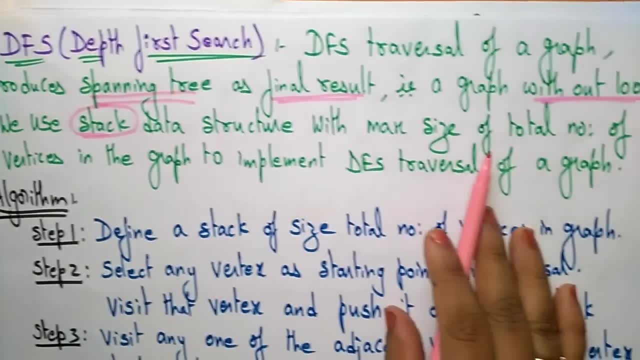 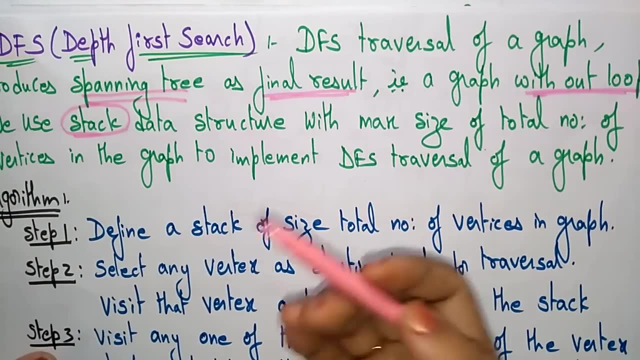 tree. so here the depth first search uses a data structure as a stack. we use stack data structures with maximum size of total number of vertices in the graph to implement dfs traversal of a graph. what it means so that status data structure stack uses a maximum size. how much of size it will be used? 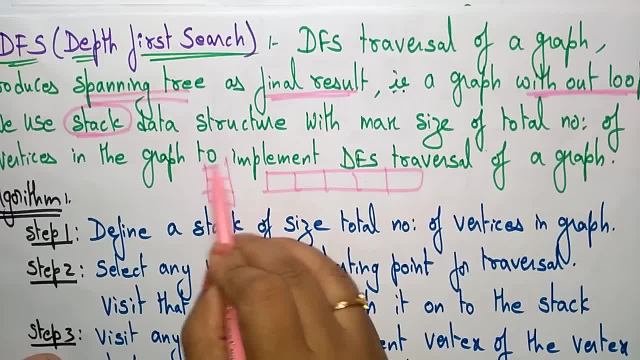 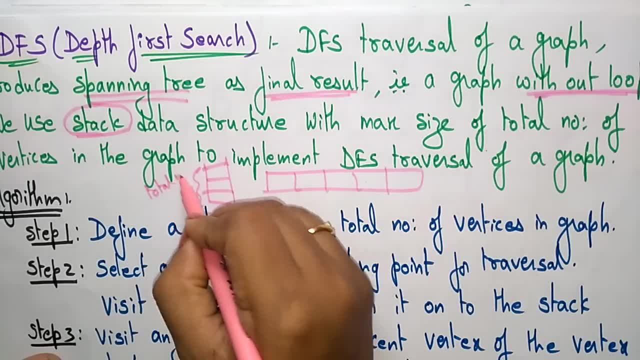 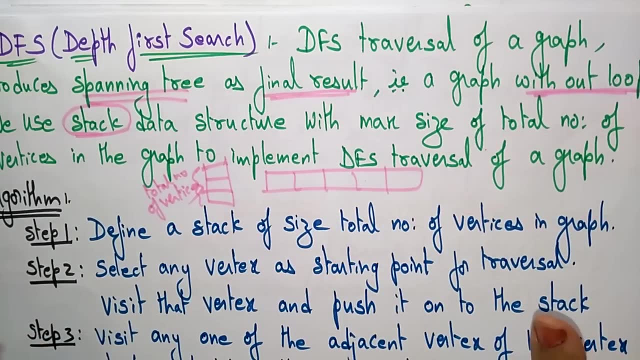 whether it is a queue means if it is a dfs means it is a stack. so the the maximum size of the stack is nothing but the total number of total number of vertices that are present in the graph. total number of vertices present in the graph is the size of the stack. first let me explain the. 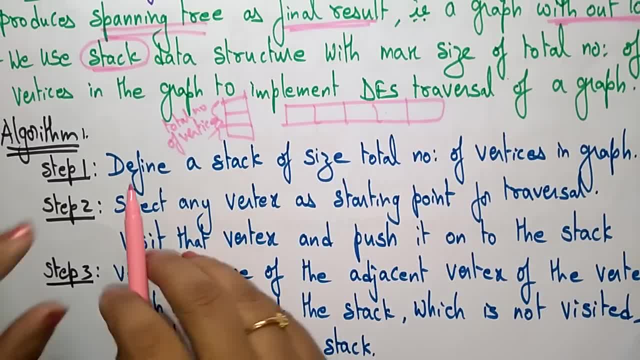 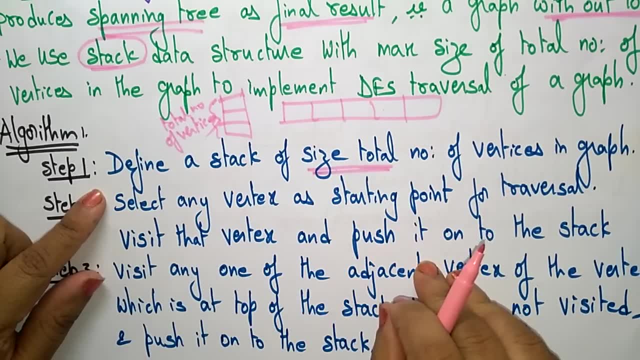 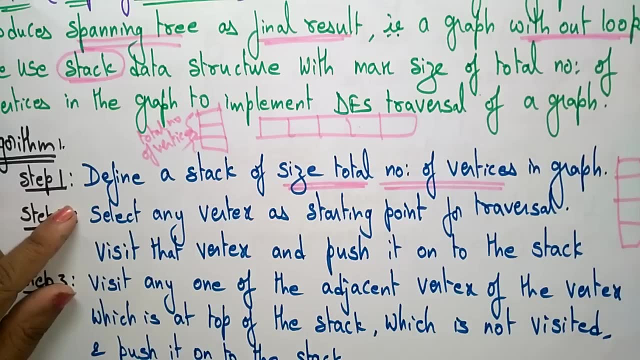 algorithm. after that i will explain with example. for example: first define a stack of size- total number of vertices. for first you have to define the size of the stack, that is, the total number of vertices, so so that you can arrange an empty stack on the memory with that particular size. after that, select any vertex as a starting point. 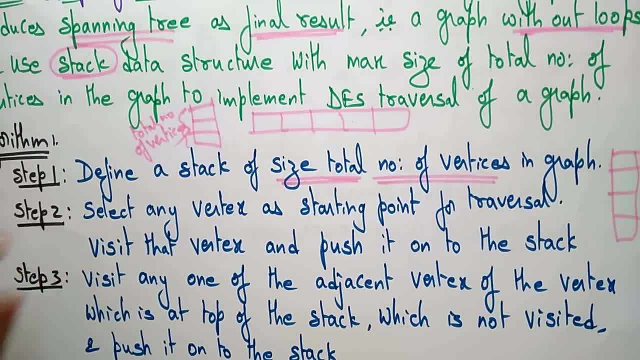 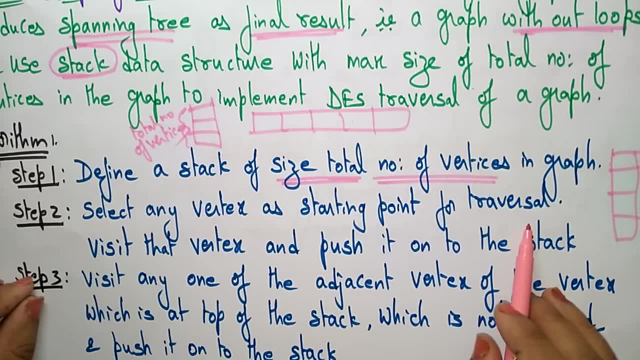 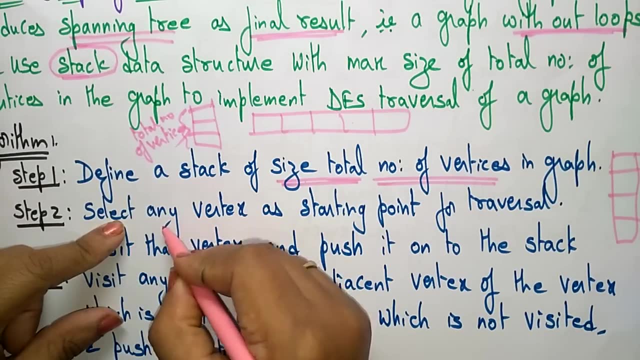 so, whatever the graph you are taking, just take any whatever it is your interest. so, based on your selection, you can visit the nodes. select any vertex as a starting point for traversal, so visit that vertex and push it in on the stack. so, whatever the vertex that you are visiting, that vertex has to be pushed onto the stack one by one. 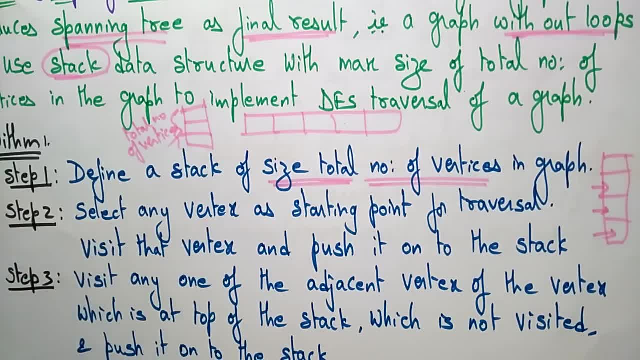 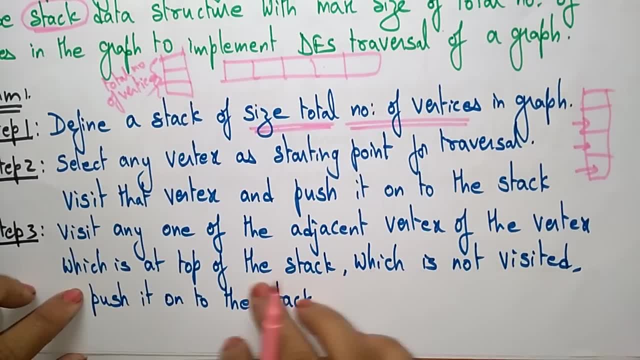 after one, the adjacent next, adjacent next, that will be pushed onto the stack. that is the second step. visit any one of the adjacent vertex, of the vertex which is at the top of the stack, which is not visited, and push it on the stack. suppose if the vertex that is 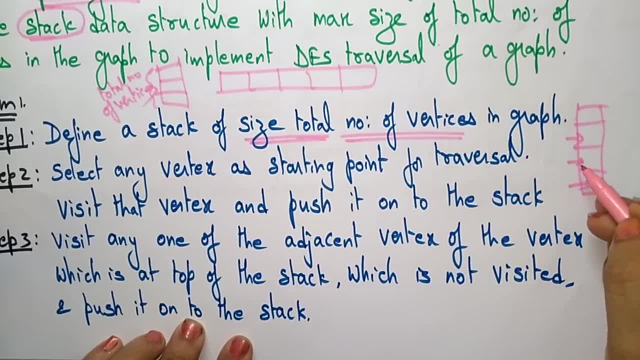 that it is not visited. you just push that vertex on the top of the stack. suppose if you visit a first, next you want to visit b. b is not visited up to now, so just put it on the stack next. if you, the adjacent vertices are b and c. here b is already visited, c is not visited, so just put it on the. 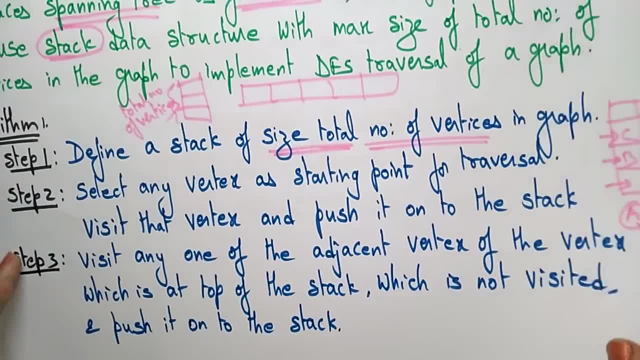 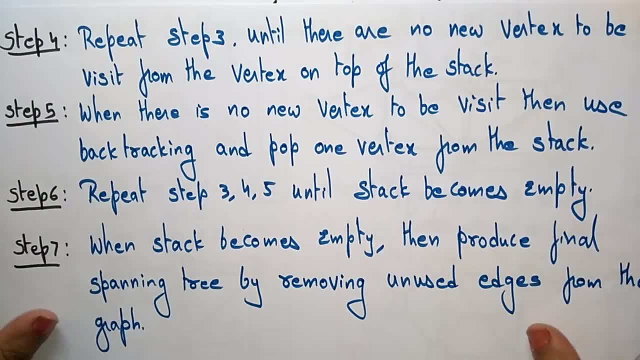 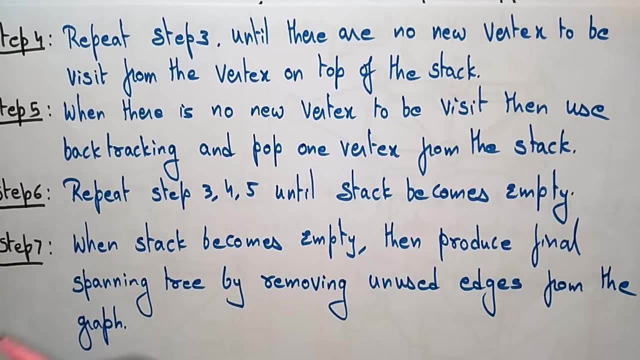 stack like that. okay, so you have to. if it is not visited, just put it onto the stack. next step, step four: repeat until there are no new vertex to be visited from the stack on top of the stack. so just repeat that step. whatever the previous step, visit the adjacent vertex and just place it on the top of the stack. 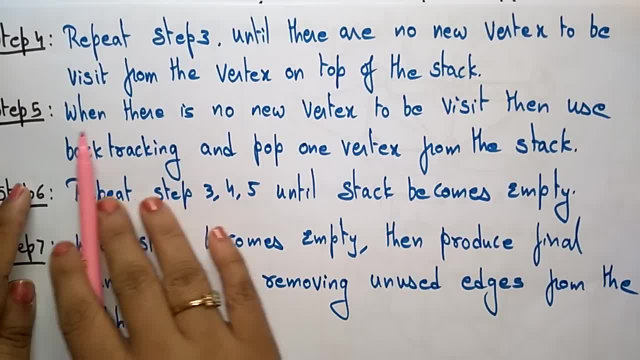 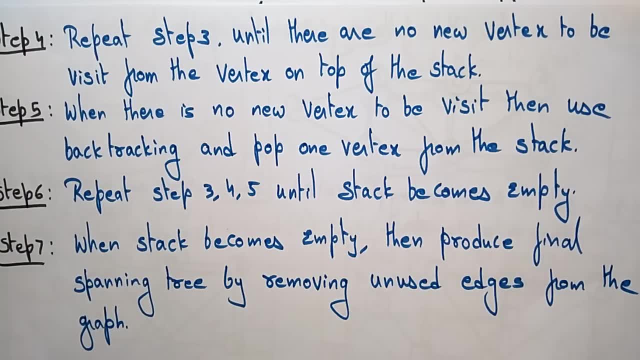 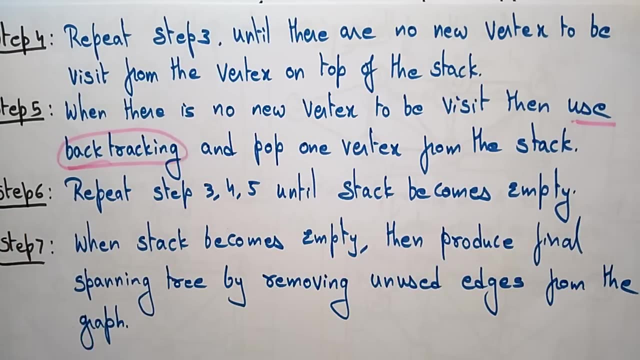 until there are no new vertex. okay, step five: when there is no new vertex to be visited, suppose if all the vertices that you are already visited, then what you have to do you just use backtracking here in the. here the backtracking will be occurred in depth. first search: 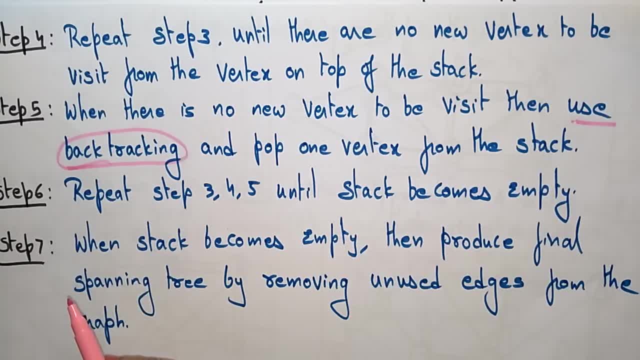 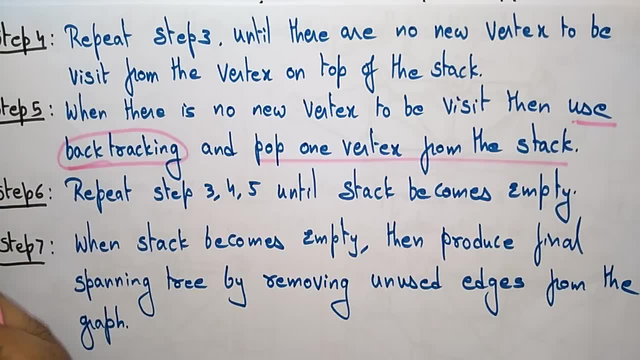 so when there is no new vertex to be visited, then use backtracking and pop one vertex from this stack. whenever you are doing the backtracking, just pop that element means delete that vertex from the stack. that is the top of the element in the stack. so repeat step three, four. 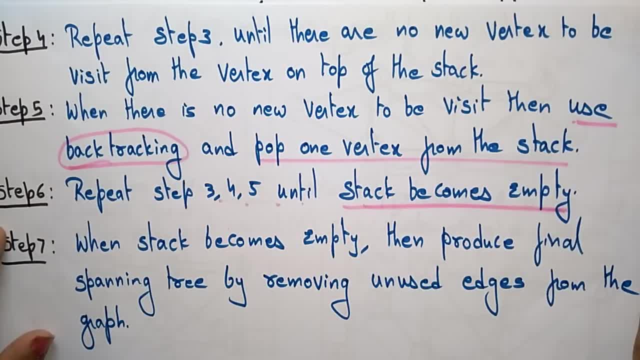 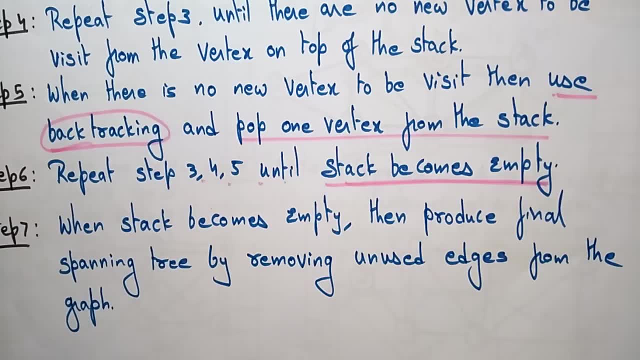 five until the stab stack becomes empty. so when stack becomes empty, then produce final spanning tree by removing unused edges from the graph. so this is a way you are going to construct the dfs graph. so first take the size of the stack means based on the number of vertices. 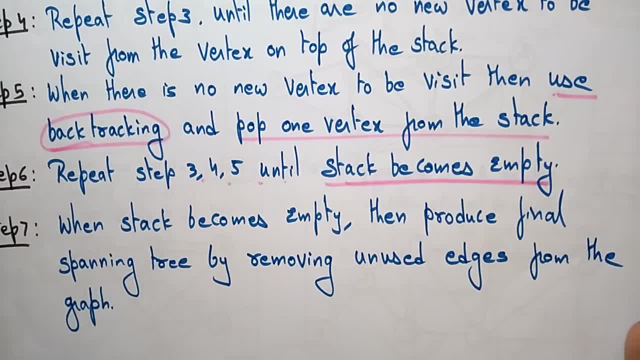 you can make the size. size of the stack. next, take any one of the vertex as a starting vertex and try to visit that first and place it on the stack next. whatever the adjacent vertices for that stack, that should be placed on the top of the stack. okay, you have to repeat until there are no. 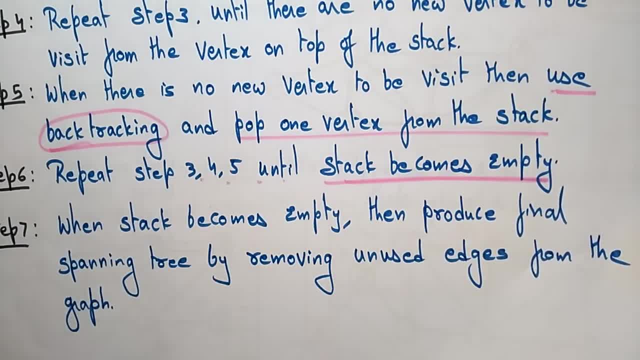 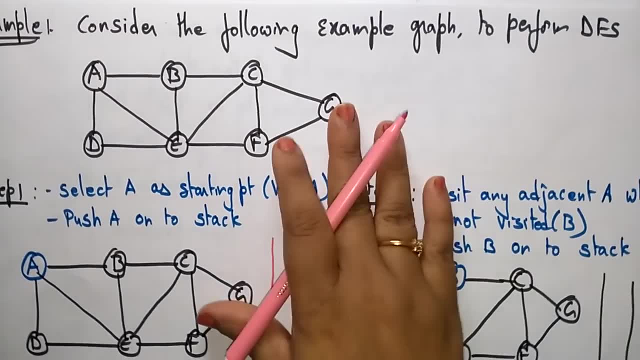 more visited vertex. okay, so in this way you have to follow the algorithm. let me explain the example, then you will understand what a algorithm is. so here i am considering the graph, which is a. i want to construct dfs, for this graph means i want to make it as a spanning. 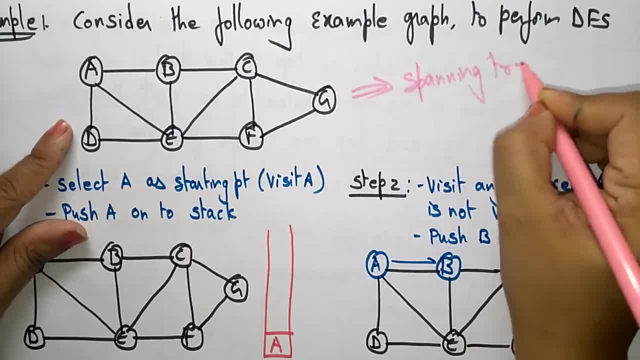 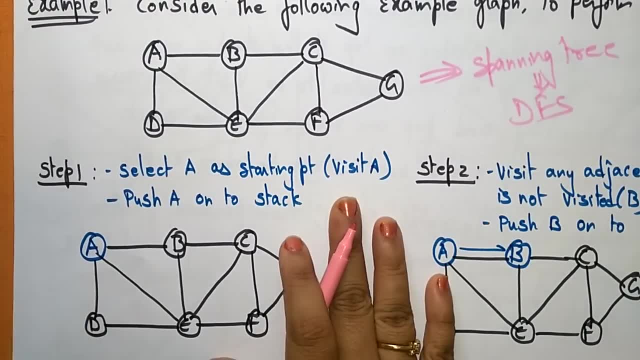 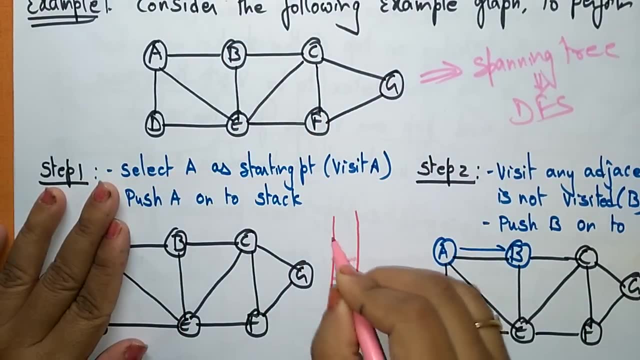 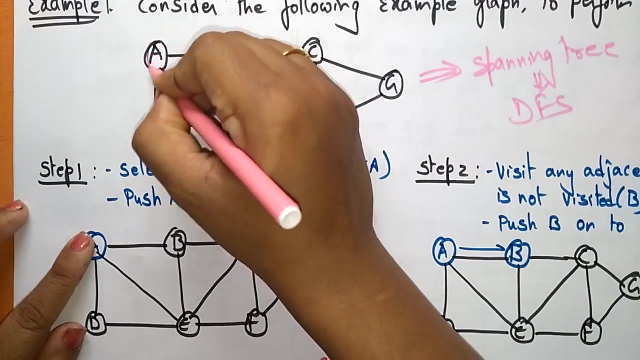 tree. the final output should be a spanning tree, which is dfs in the form of dfs. so step one what i said, according to the algorithm. so here the stack consists of one, two, three, four, five, six, seven. so seven spaces will be there in the stack. first, select a as a starting point. so here i am selecting. 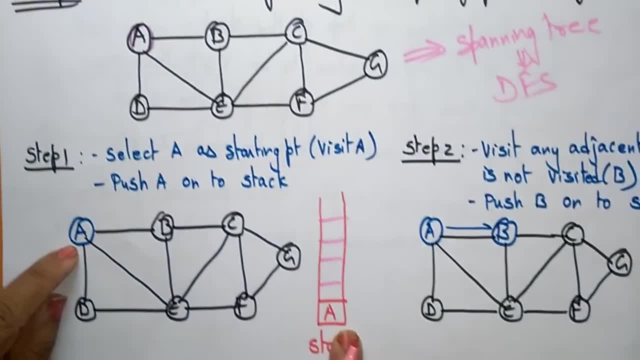 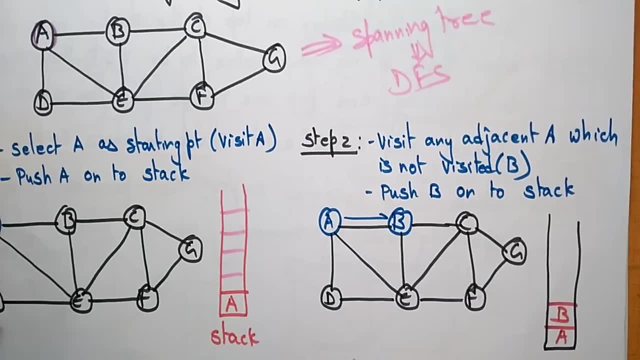 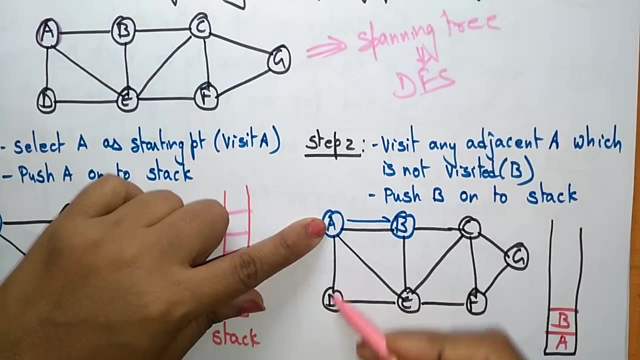 a as a starting point and push on to the stack next in step two: visit any adjacent of a. so whatever. take only one vertex now, okay, which is not visited. that should be compulsory. visit any adjacent of a: either you visit d or e or b, based on your interest, okay, but you have to make sure. 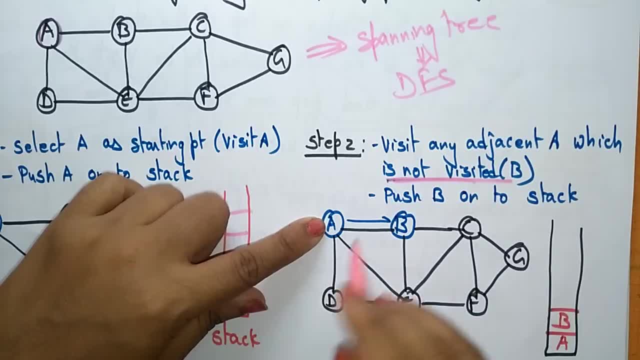 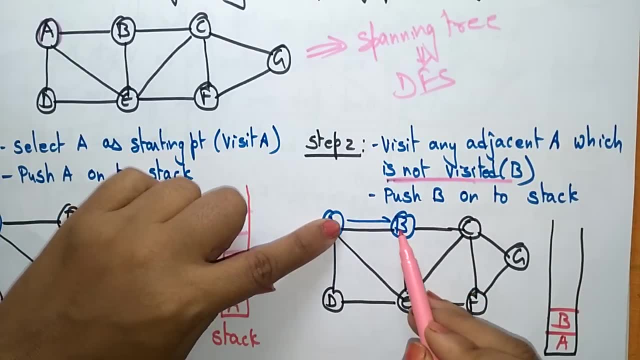 which is not visited, that you have to be take. so here b, d e, no one was uh taken into up to now. we didn't take any vertex now, so just i'm taking b and i'm pushing on to the stack top of this stack. next step three. 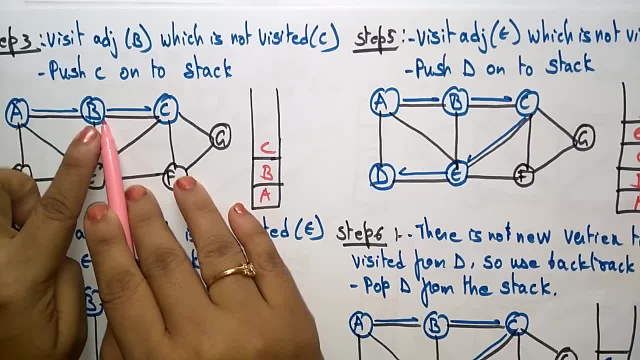 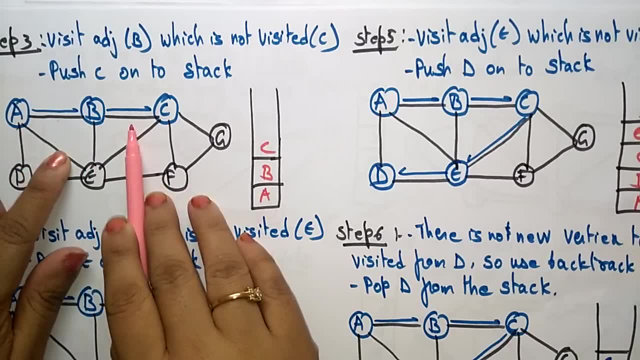 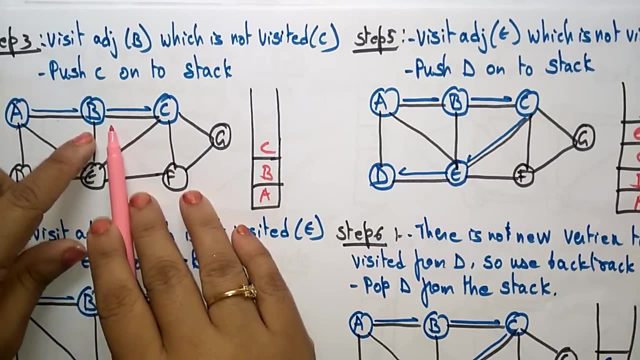 next visit adjacent b. so now i'm visiting b, which is uh. what are the adjacent vertex of the b? the b adjacent vertex are e, a and c. so here a is already visited, c is already visited and uh- sorry, uh, a is already visited, uh, so the 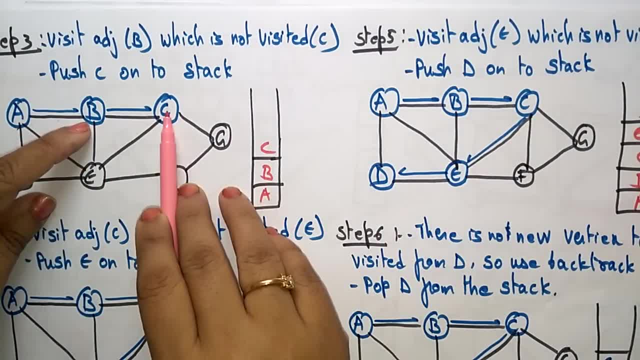 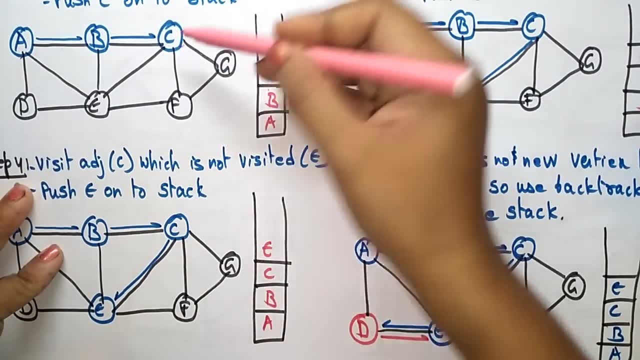 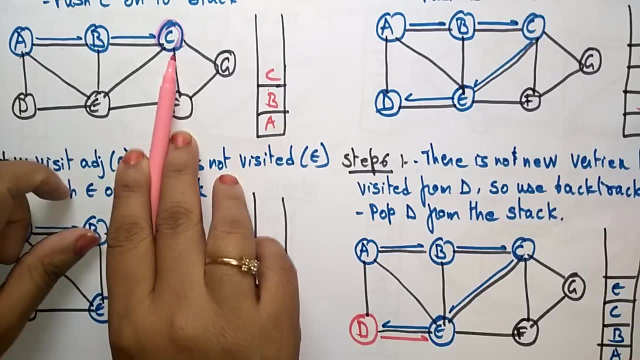 adjacent of b, which is not visited, is either e or c. so just after b, i'm just placing c onto the stack. okay, now coming to the c. so this is the top of the stack now. now coming to the c. visit adjacent c, which is not visited. so from c, which is not visited, e, f, g are not visited. b is already. 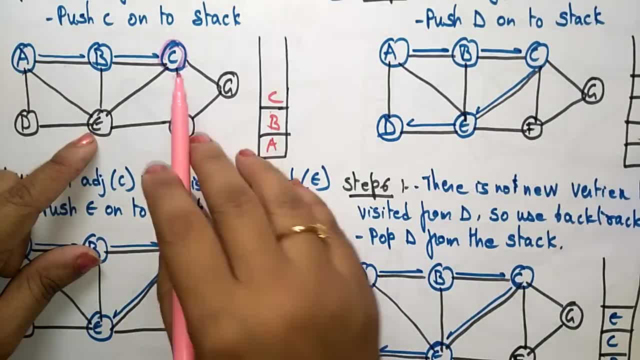 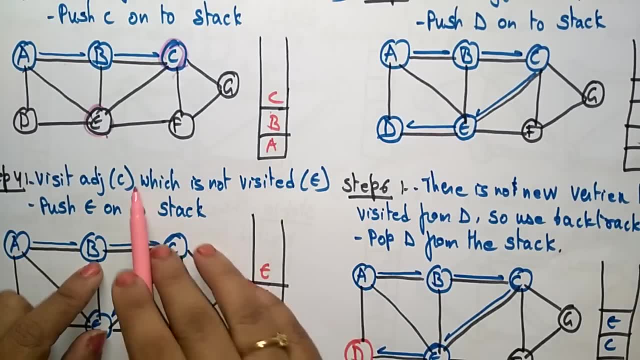 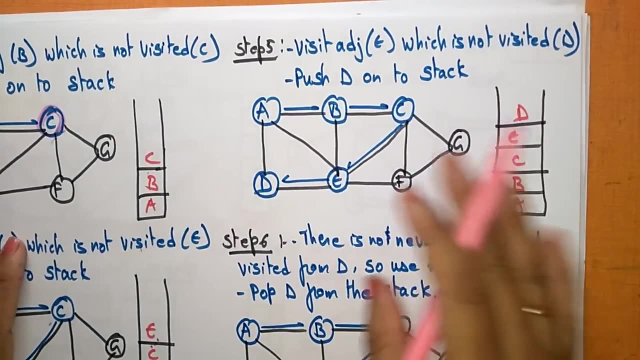 visited. so from this i'm taking according to the alphabetical order. so now i'm taking e. so just place e on the top of the stack. now adjacents of c, which is not visited, is e, so that i am push onto the stack now. coming to now, the top of the stack is e. so visit adjacent e. 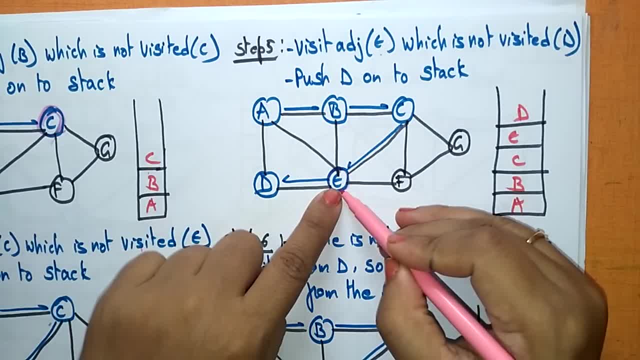 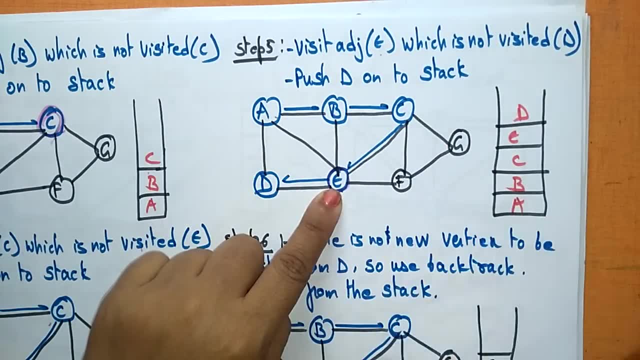 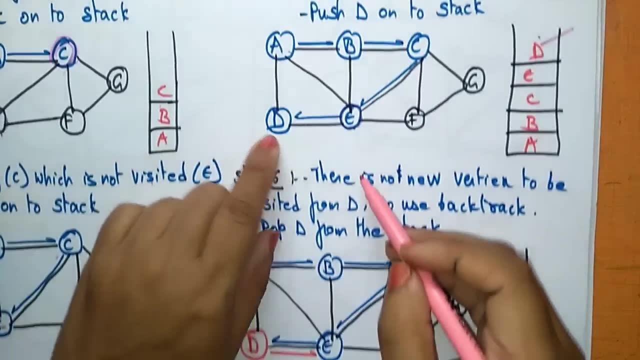 which is not visited. so the adjacent of e, which is not visited, is okay here. a- i already visited. b already visited. c already visited. f and d are not visited. so according to alphabetical order, i'm placing d on top of this tag now coming to the d, so d is the adjacent vertex now. 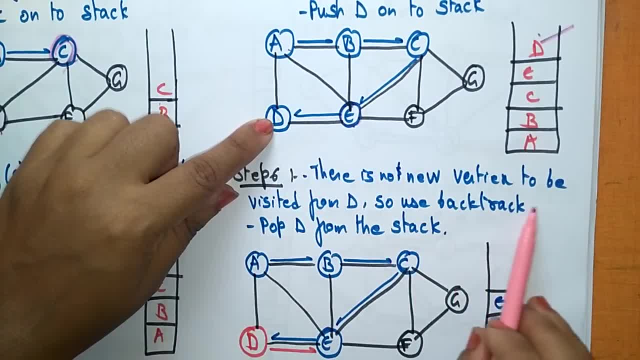 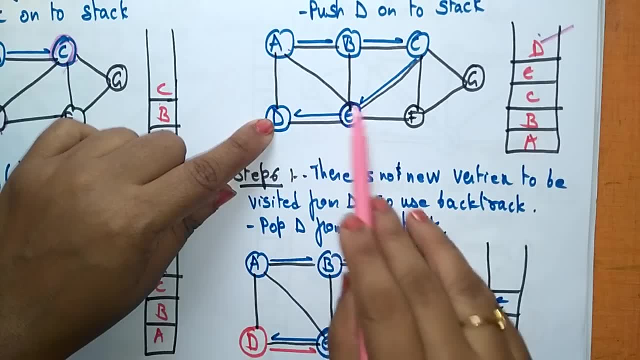 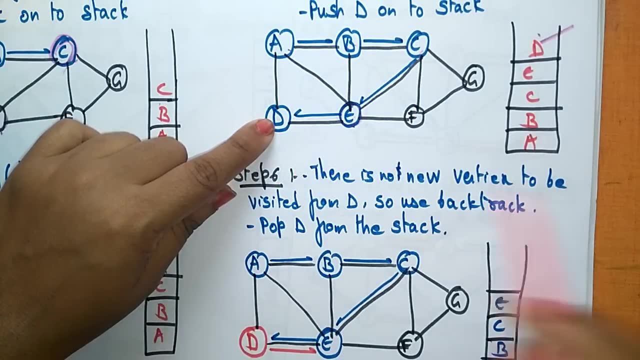 d is the adjacent vertex. check here: there is no new vertex to be visited from d, so from d, a is already visited, b, e, c, so i'm already visited vertex. i'm placing as a blue blue circles. so a, b, c, e is already visited. so there is no new vertex to be visited from d. so what i have to do, i have. 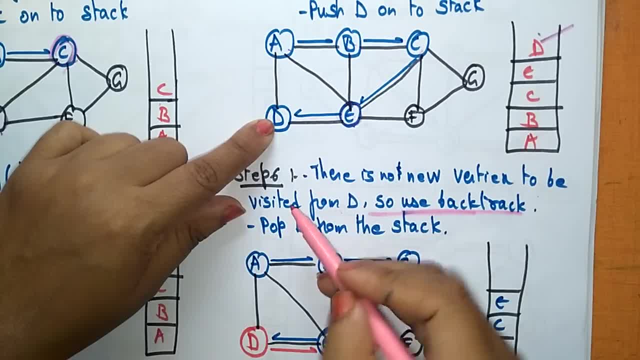 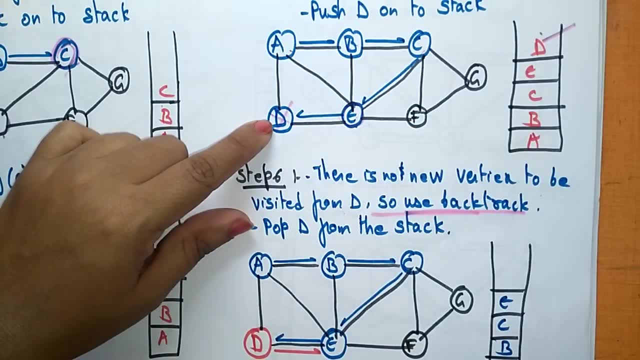 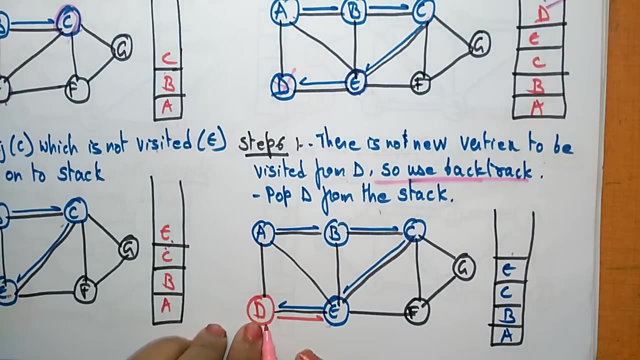 to use the backtracking. what i said. according to the algorithm, whenever you are performing backtracking, try to pop the element from the stack. so just delete the d element from the stack. come back so that i marked it as a red color. so i'm coming back now. check from e. so what are the 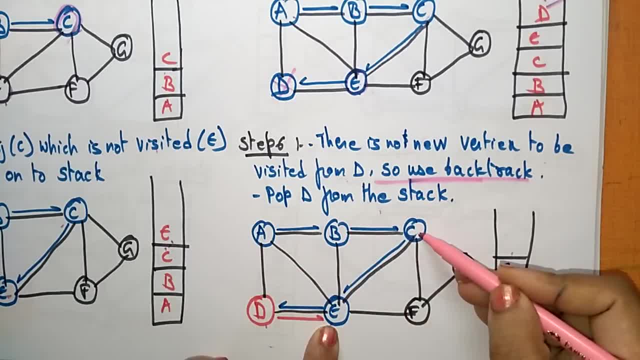 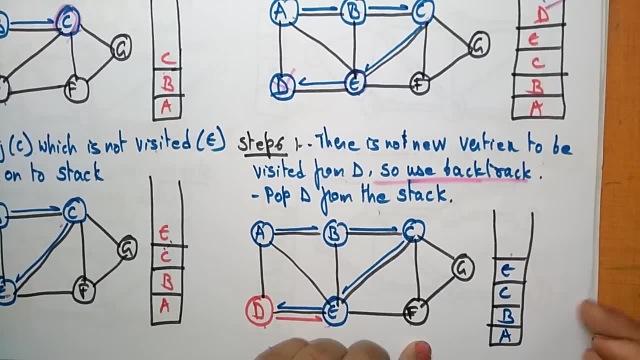 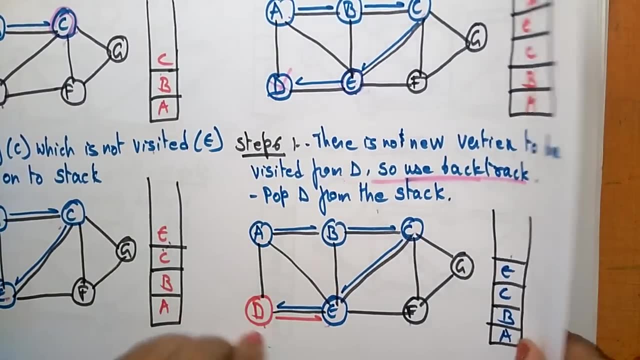 adjacent vertices of e, d, a, b, e. okay, the vertex that it is no up to now we didn't visited, is f, so which i placed as a black. the visited vertices: i make mark it as a blue and the deleted from the stack: i mark it as a red color. 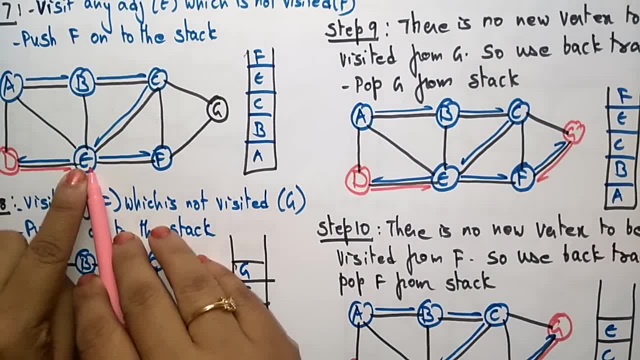 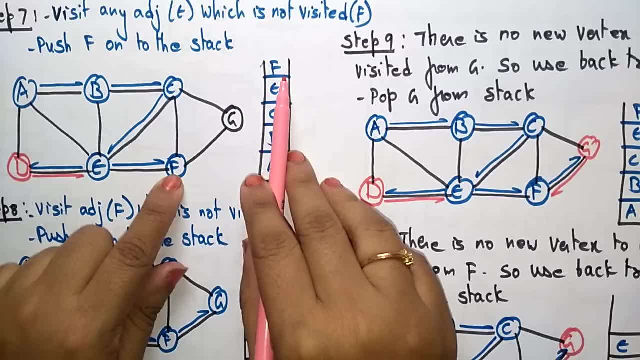 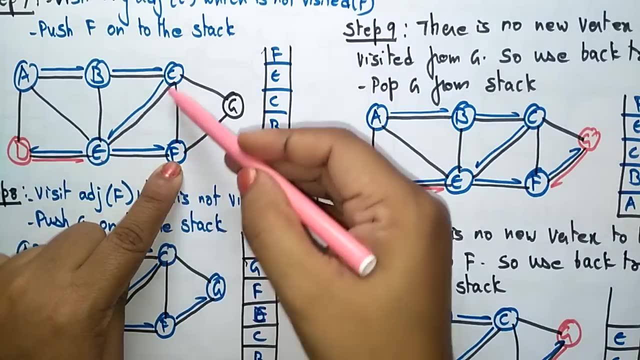 so visit any adjacent vertex of v which is not visited. so up to now, which is not visited is f. so f is placed on the top of this stack. now, coming to the top of the stack, which element f? now check from f, which are the adjacent vertices, which are the adjacent vertices of f, or e, c, g, so from: 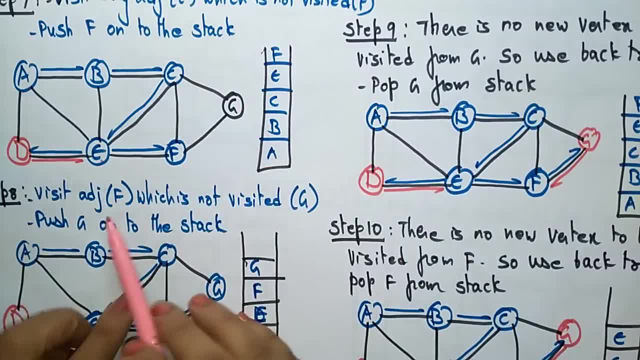 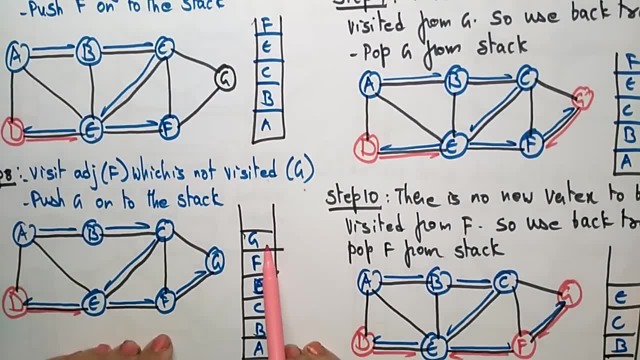 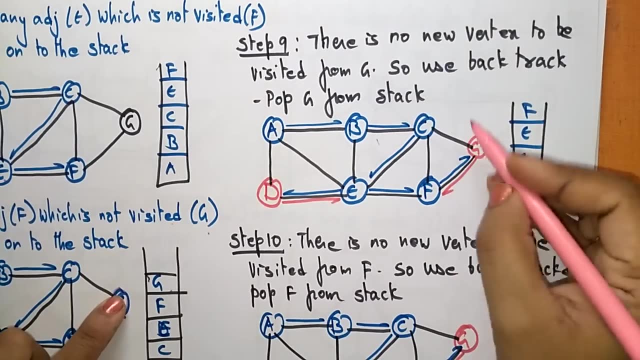 all these three. g is not visited up to now, so we visit adjacent f. which is not visited is g. so just push u g on top of this stack, now stack. okay. so now coming to the g, that just take the top of the stack. so whenever i take the top, 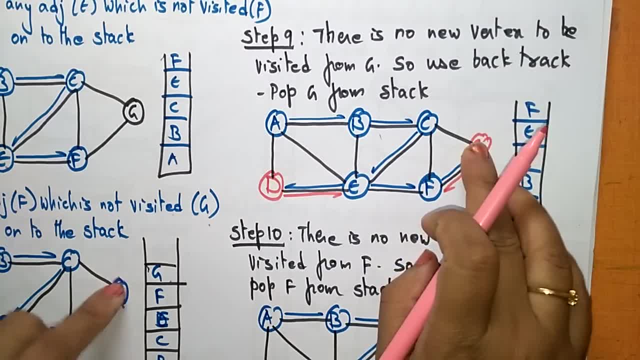 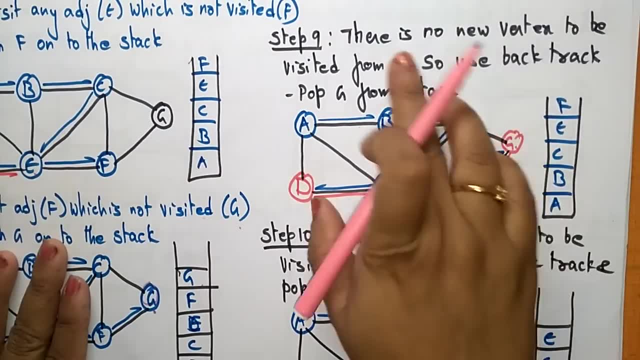 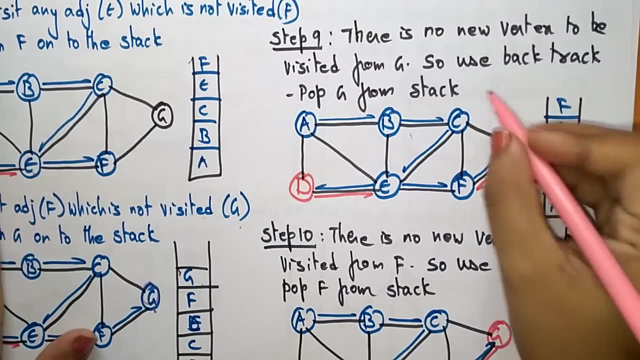 of the stack. i'm checking now from g- all vertices. or i'm visited a, b, c, d, e, f, all vertex i already visited. so there is no new vertex to be visited from g. so what i have to do? so whenever there are no vertex to visit, you just use backtrack. so whenever i'm backtracking. so from f to g, i came. 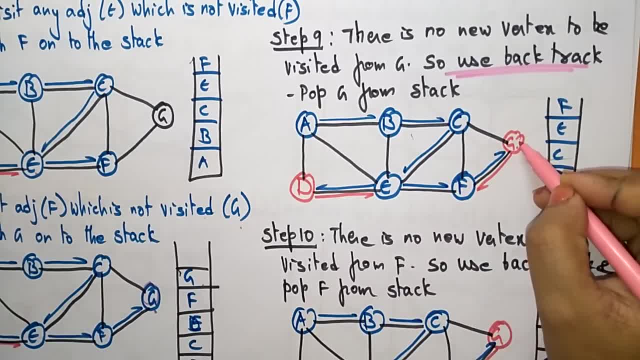 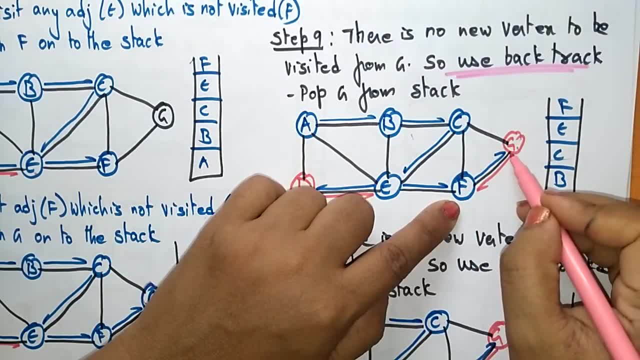 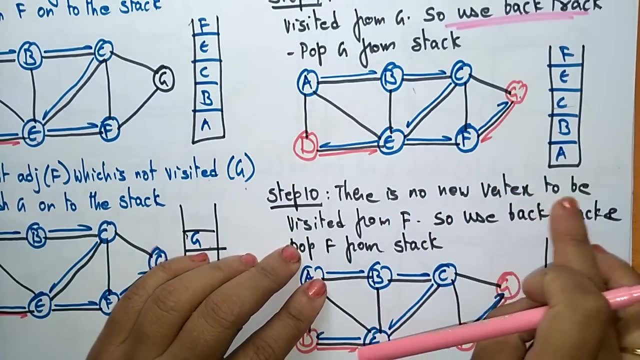 uh from f. uh, the adjacent i had, f has taken g as a adjacent vertex, so i just use backtracking. so, backtracking, whenever you're doing backtracking, just pop the element so the g will be popped from the stack next. from f. there is no vertex to be visited from f, so use backtracking and pop f so. 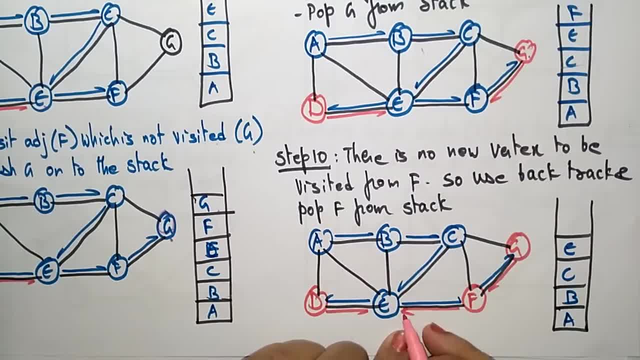 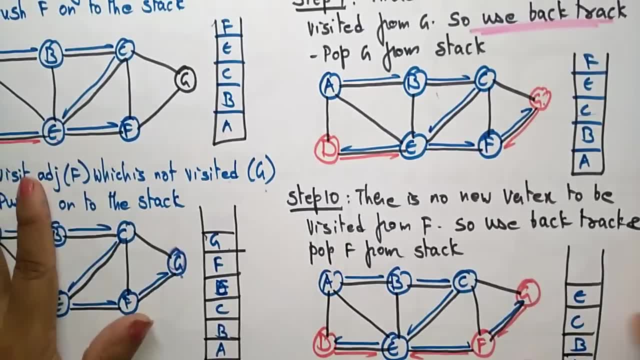 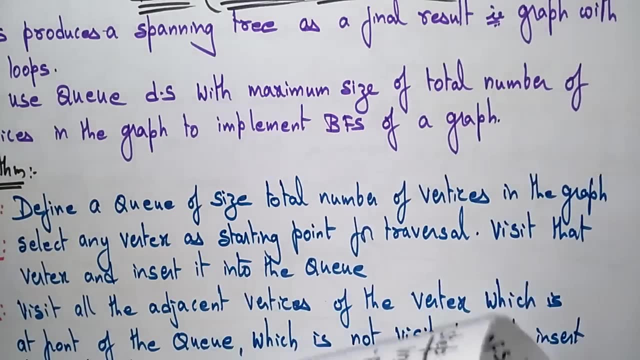 this time. so this time. so this time, just pop f also. so just backtracking. so where it is come, it's just backtracking. now pop f. now. e is the adjacent vertex. now check from e which vertex is up to not visited, so that we have to be checked. 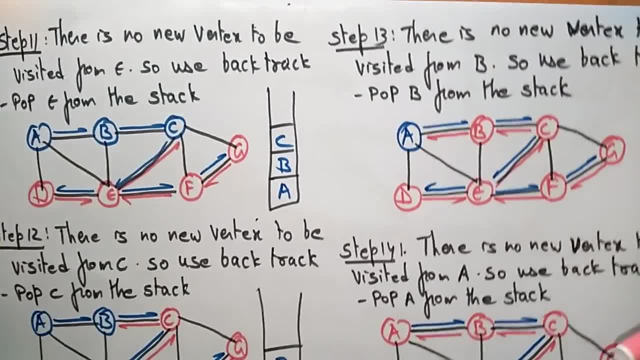 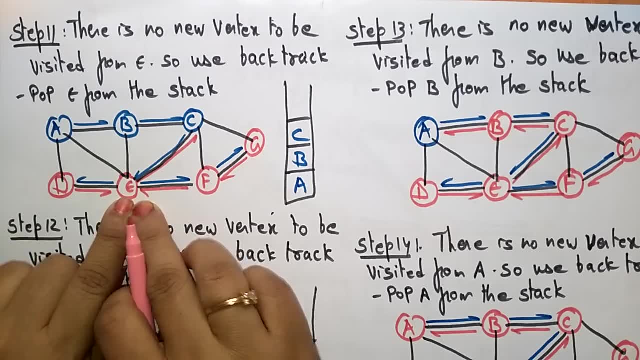 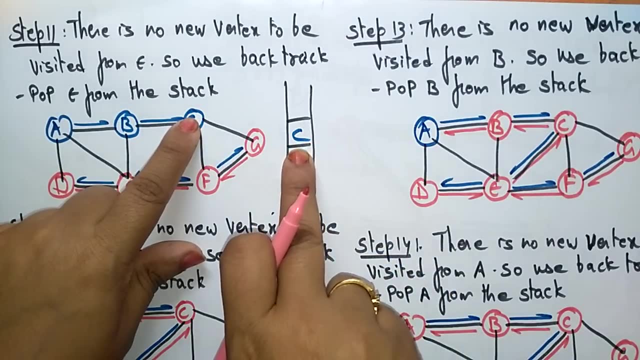 so there is no vertex to be visited from e, so use backtracking. so where i had to go, okay, so the backtracking. so from c to e we came. so just backtracking. so pop the e element. so after c the top of the stack is c. so all vertex already. 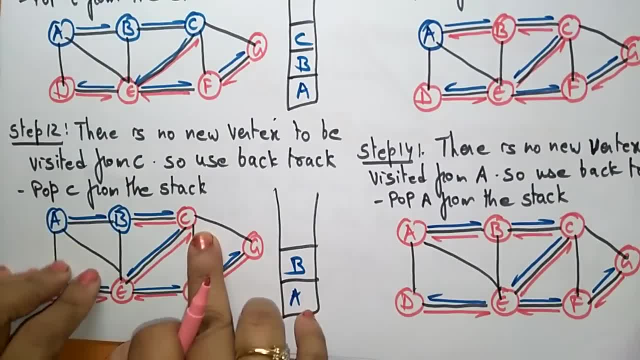 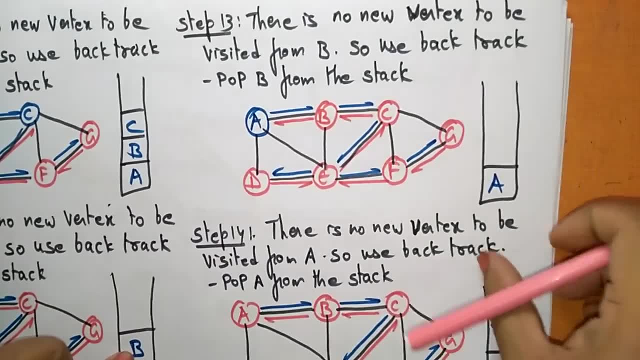 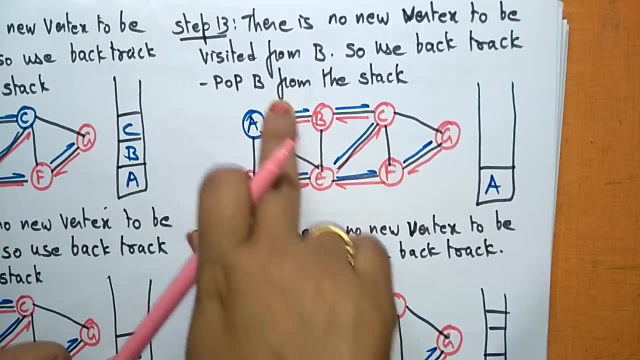 visited, so use backtracking. then pop c, so this time c was deleted from the stack. next the extent of c: uh. next is b. there is no new vertex to be visited from b, so use backtracking. and again we reach the starting element. so just traversal from start and, uh, backtracking. so just backtracking. 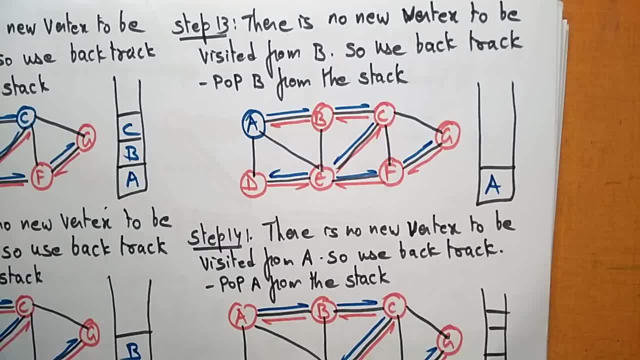 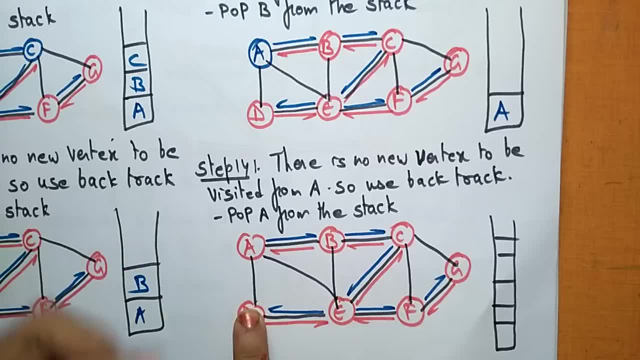 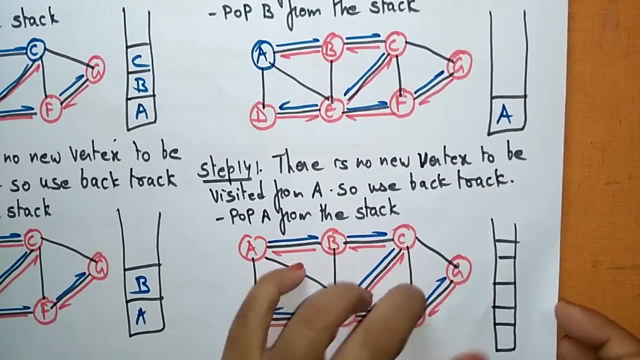 uh, came back using backtracking to reach again the a. so there is no new vertex to be visited from a, so use backtracking and pop element so to buy to perform backtracking. there are no vertex to be backtracked, so just pop the element from stand. so now the stack becomes empty. so the stack became.